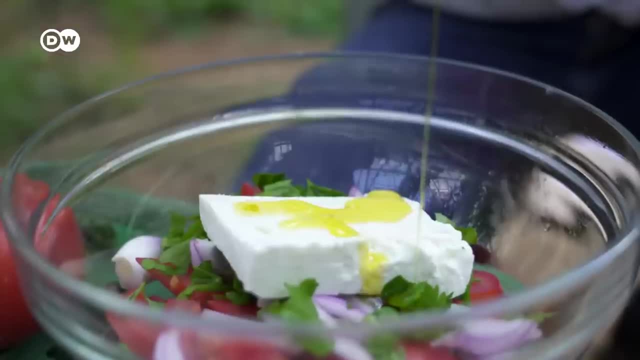 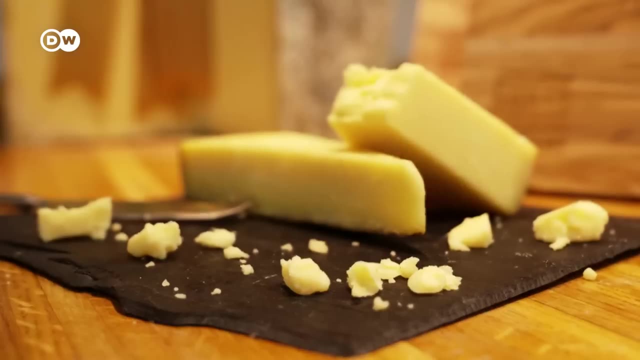 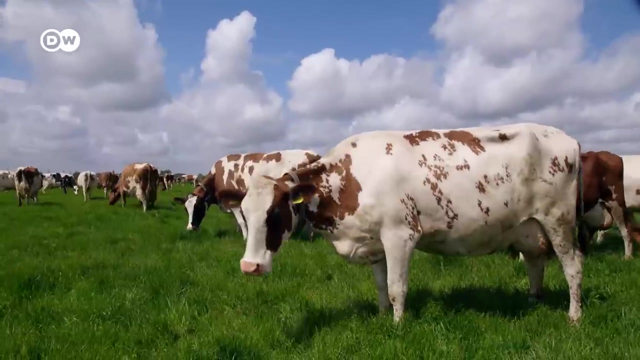 We really hope you like cheese, because that's what this video is all about. We present five classic European cheeses that you simply have to know. Say cheese. We start out in the Netherlands, home to one of the best-known types of cheese: Gouda- a special variation of it. 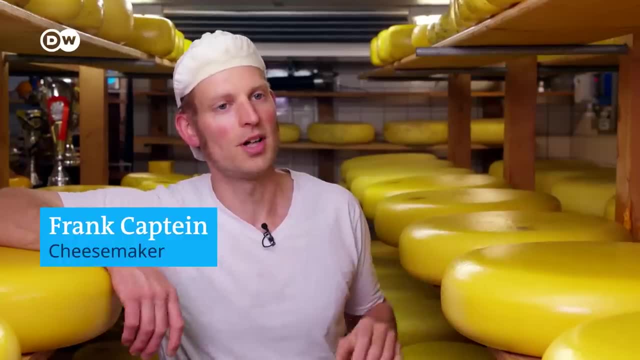 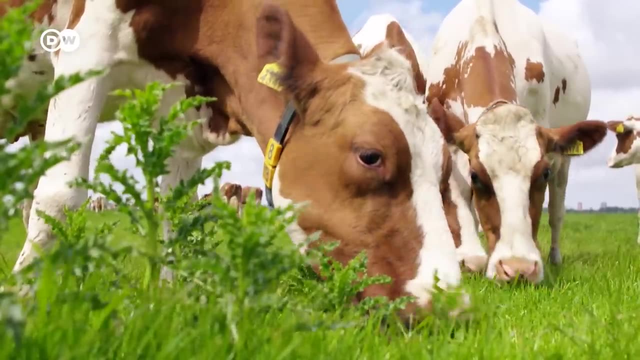 Boeren Gouda cheese. Boeren means farmer, and special about it is that Boeren Gouda cheese is a cheese produced on the same farm as where the cows are milked, and we don't heat the milk, so we produce cheese from raw milk. 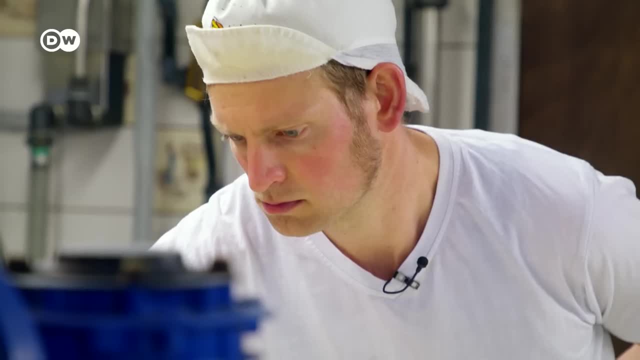 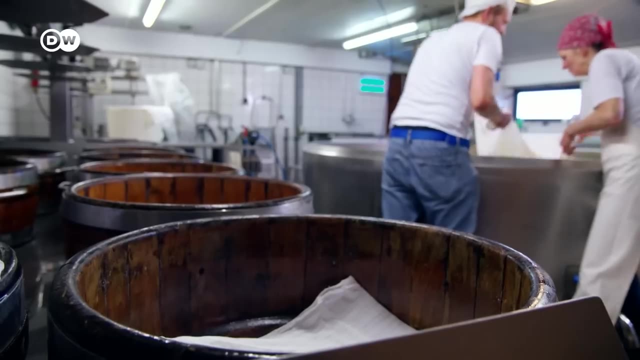 Besides the raw milk, lactic acid, bacteria and rennet are the main ingredients. Rennet is an enzyme from the stomach of calves that curdles the milk. The curdling separates the whey from the cheese curd, which then goes into wooden. 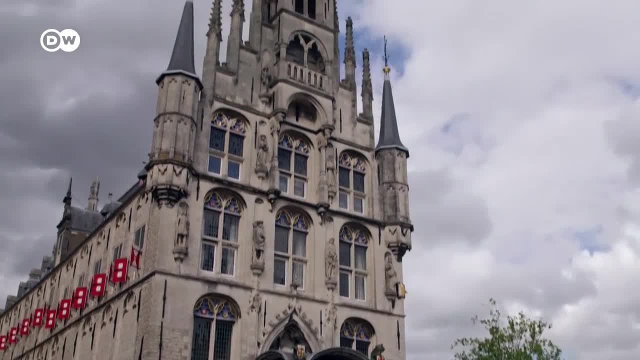 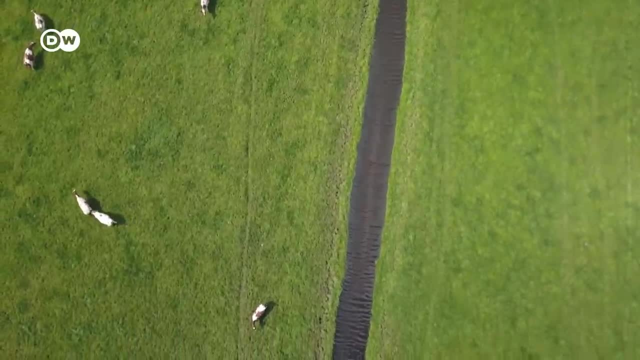 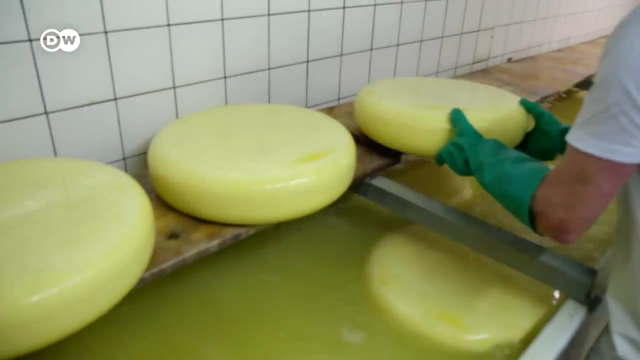 curds. Gouda, by the way, is a town in the Netherlands. It's surrounded by green meadows, so the natural thing to do was buy cattle, let them graze and make the namesake cheese from their milk. After the first 24 hours, the Gouda is soaked in brine. 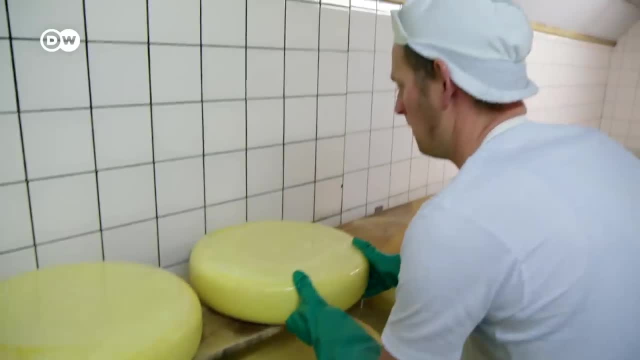 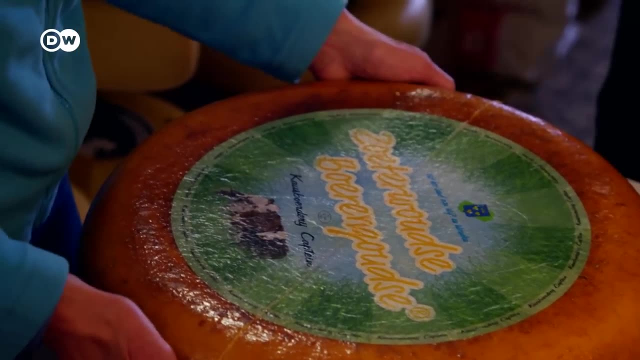 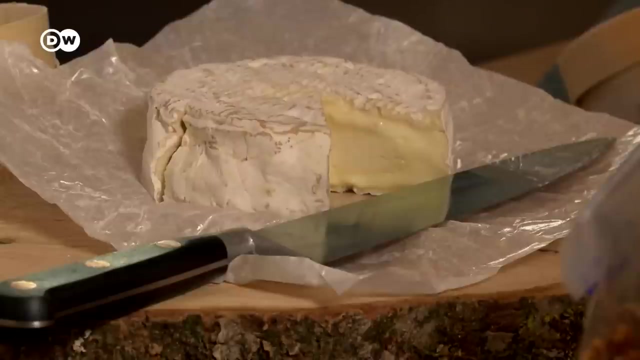 That creates the rind that protects the cheese from mould, among other things. Gouda matures anywhere from three months to several years, giving rise to variations in flavour, But all of them taste great, with bread Moving down the coast to Normandy in northern France. 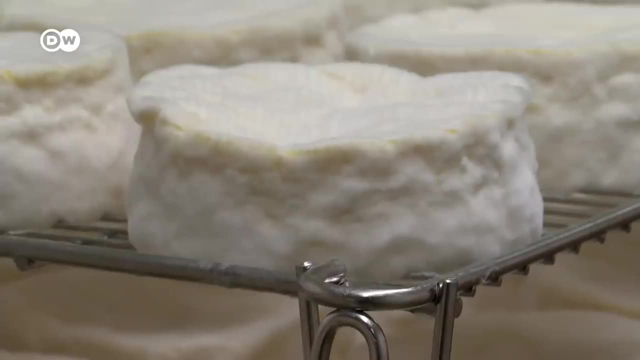 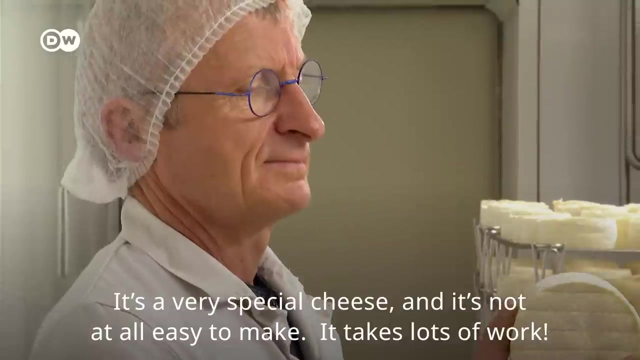 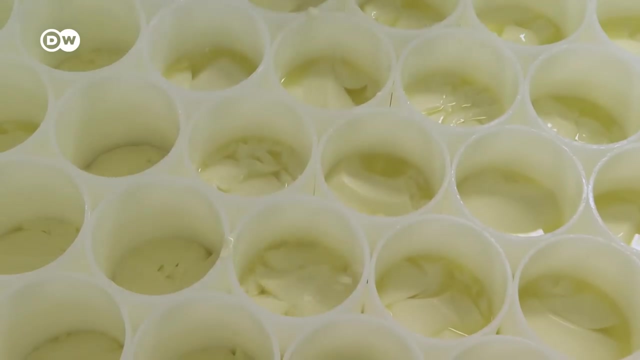 we probe the mysteries of a tasty, soft cheese. The camembert is very attached to the image of France abroad. It is special, it is complicated to make, it requires all this energy, all this observation. It's vital for the camembert to be turned by hand five times every 40 minutes. 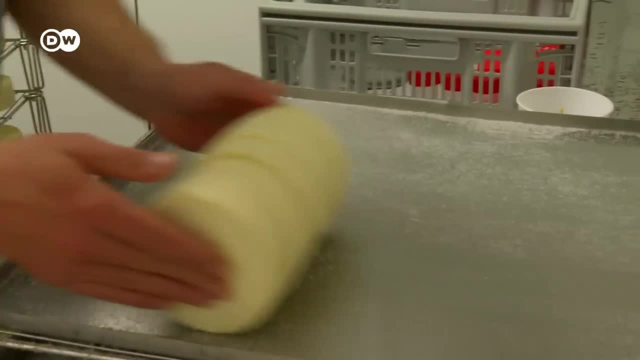 The next day salt is added. Otherwise, the characteristic of the camembert is to add salt. The next day, salt is added. Otherwise, the characteristic of the camembert is to add salt. Otherwise, the characteristic of the camembert is to add salt. 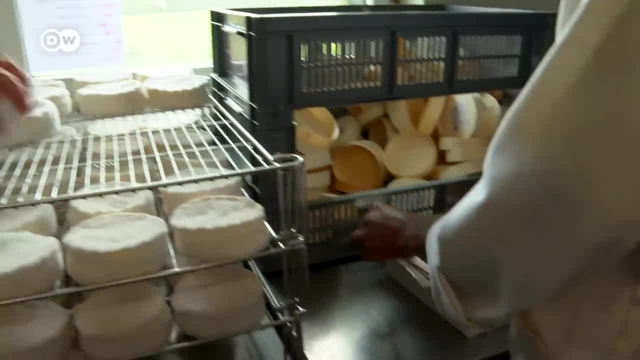 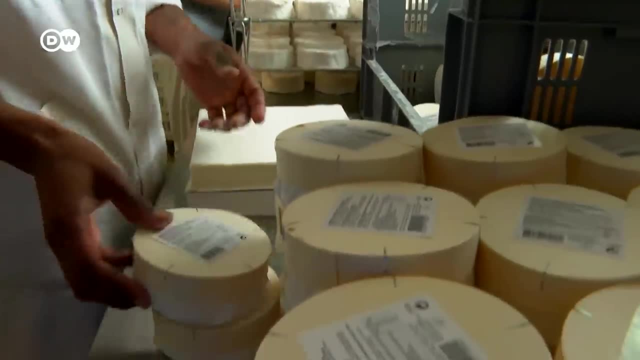 The edible mould rind wouldn't form. It ripens for 14 days before it's packed in wooden boxes to mature for one more week. It's the wooden boxes that helped carry the original camembert to success. They made transport easier. 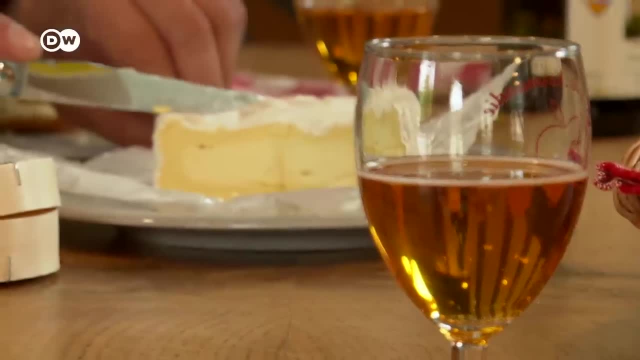 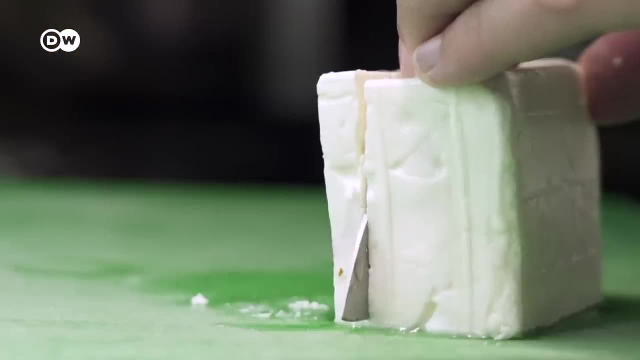 One tip. camembert is at its best at room temperature, And it's an ideal accompaniment to cider or apple wine, And it's an ideal accompaniment to cider or apple wine, And it's an ideal accompaniment to cider or apple wine. 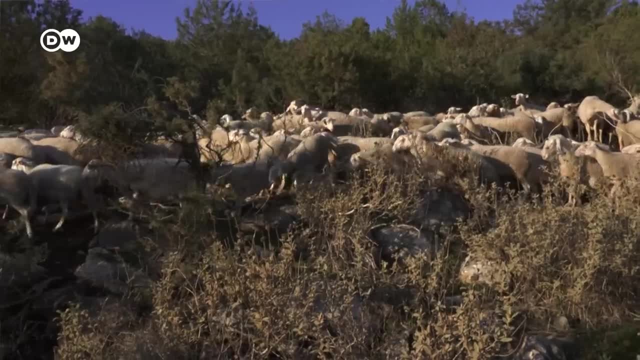 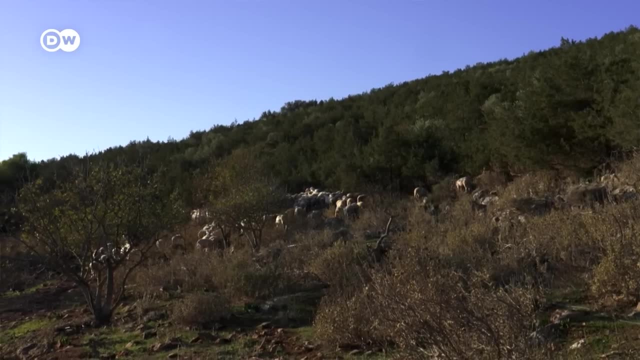 The next stop is Greece, home of the renowned feta sheep's milk cheese. Its secret lies in the rich milk from sheep that graze on lots of herbs like oregano, thyme, mint and sage. It takes three or four litres of milk to make one kilo of cheese. 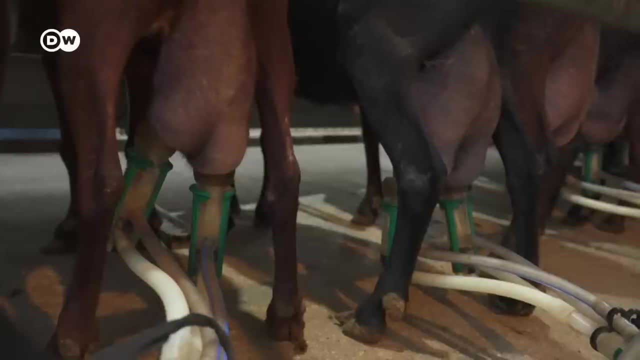 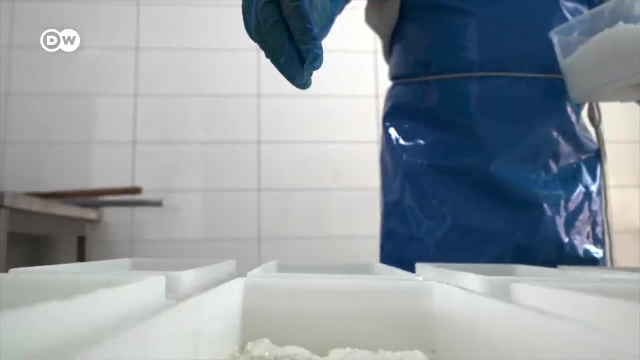 Genuine feta is made of 100% sheep's milk or at most 30% goat's milk. The sheep's curd is put into perforated moulds that let the excess liquid drain away. Salt protects the feta and lends it the characteristic taste. 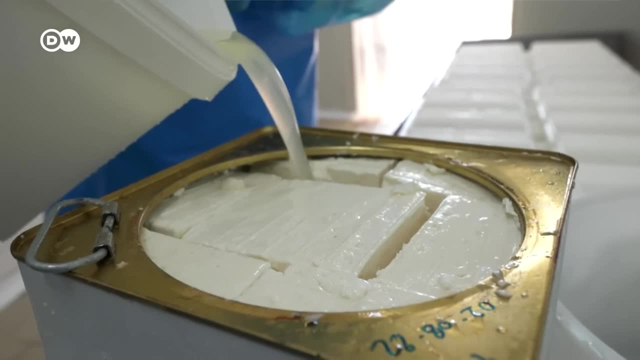 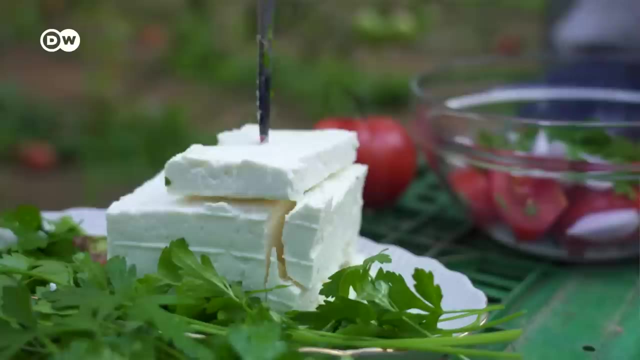 It's cut and aged in brine-filled barrels for about 15 days, then moved into cold storage until it can be brought to market. It's only allowed to carry the name feta if it's been made in mainland Greece or on the island of Lesbos. 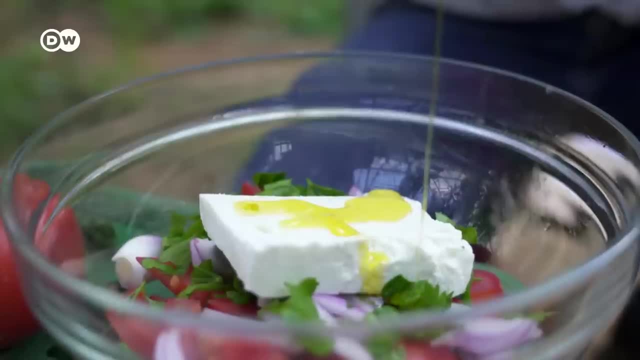 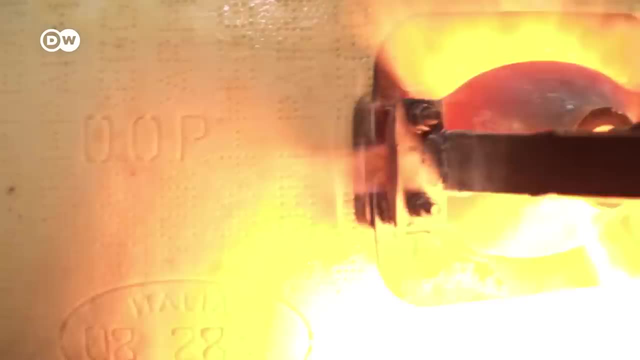 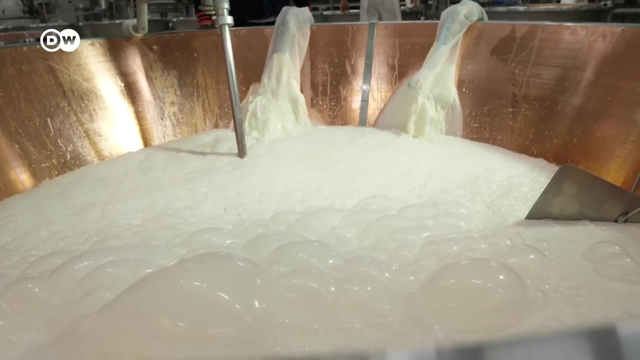 Only then is it the original feta. We putt across the Adriatic to Italy for a pinch of parmesan or, to be exact, parmigiano-reggiano. This hard cheese may be only made with cow's milk from five regions of northern Italy. 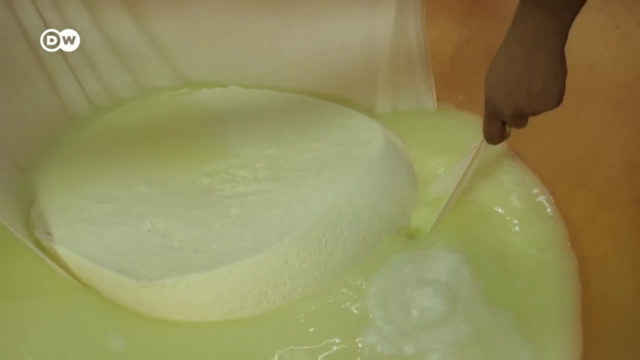 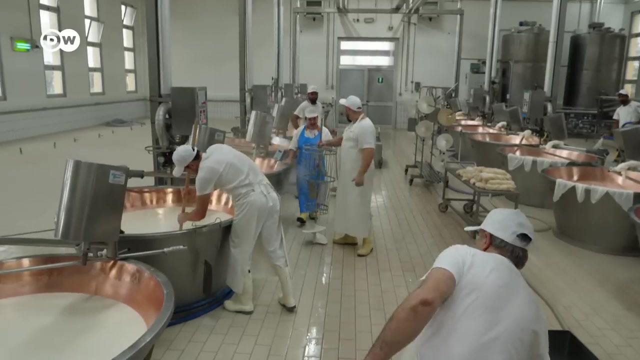 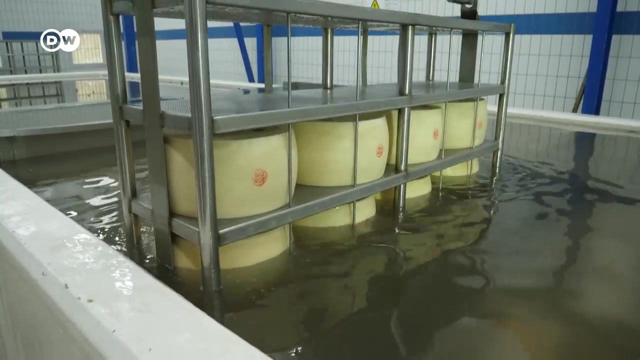 It takes about 15 litres of milk to produce one kilo of cheese. In copper vats, the curdled milk forms 80 kilogram wheels. These are cut in half and pressed into moulds. Finally, they're placed in brine for 20 days to draw the moisture out. 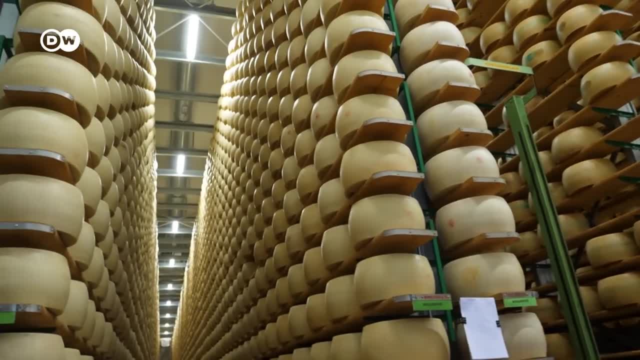 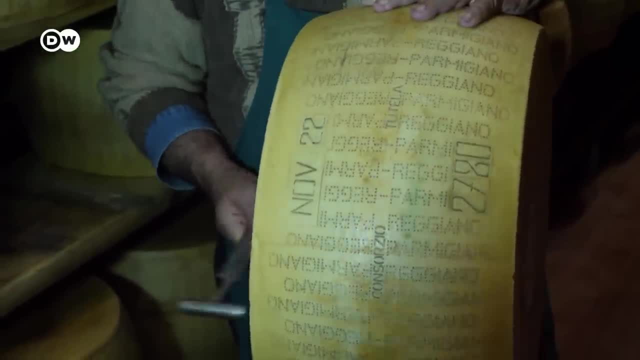 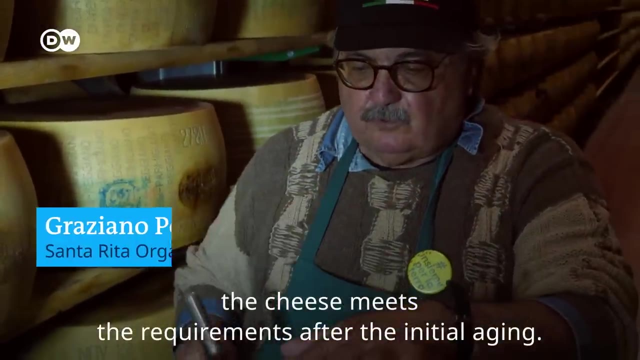 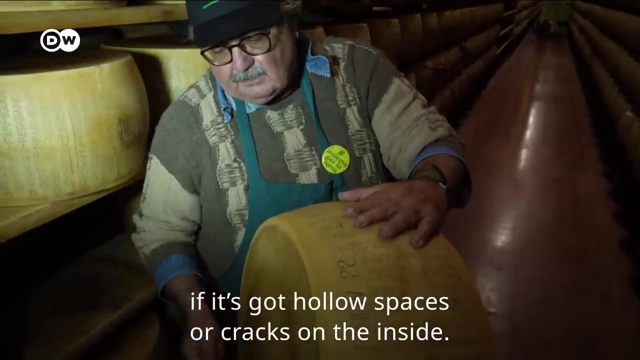 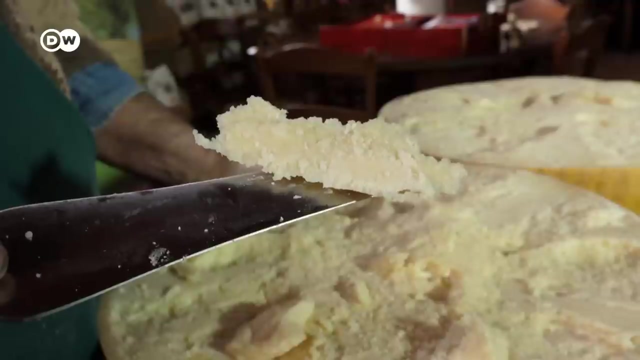 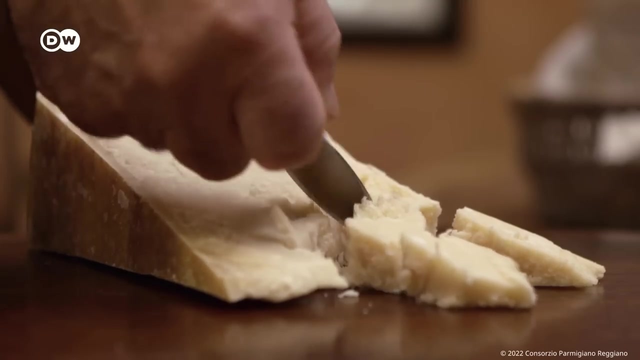 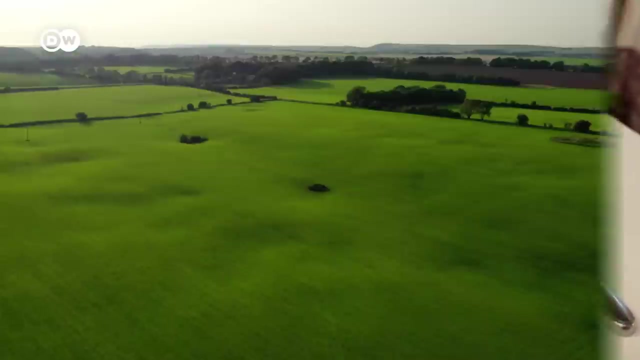 The cheese wheels mature for at least 12 months in spacious halls. Tapping each wheel with a special hammer tells about its quality. The cheese is also produced without any impurities or impurities. Even though Parmesan is a milk product, it contains no lactose. 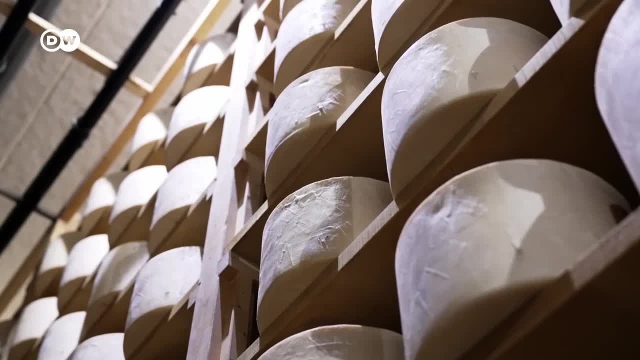 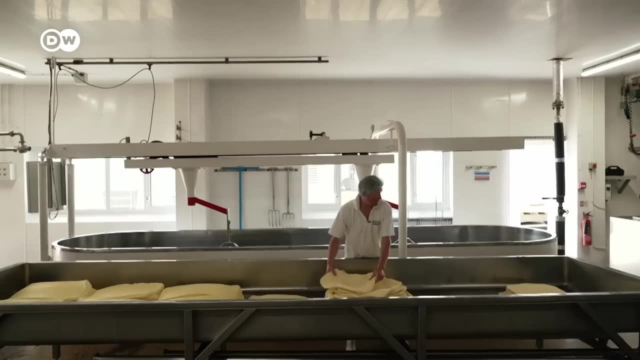 An interesting fact: Even though Parmesan is a milk product, it contains no lactose- one of the most widely sold cheeses in the world. To draw the moisture out of the cheese, it's cut into blocks. Then comes the cheddaring process.